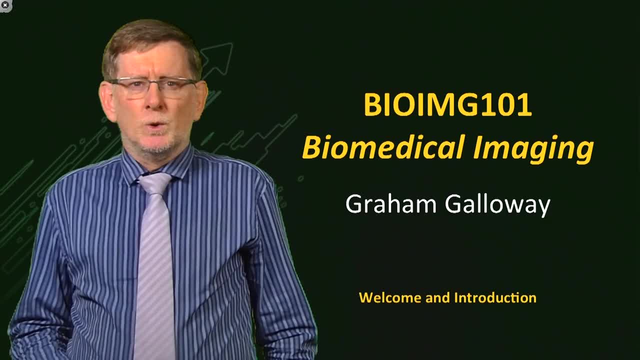 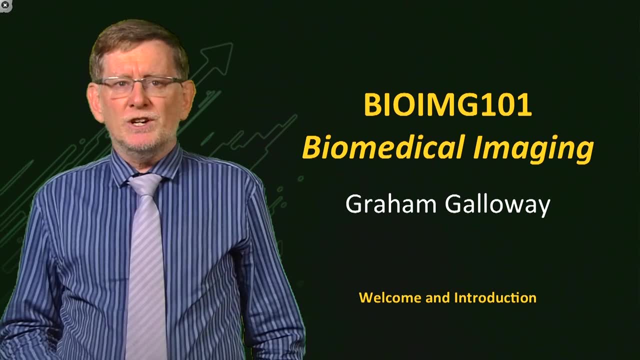 Welcome to EQX's course on biomedical imaging, in which we will introduce you to the major imaging modalities in clinical medicine. You will be taught by a team of imaging professionals who do research into new ways of using imaging to get detailed information about the human body. 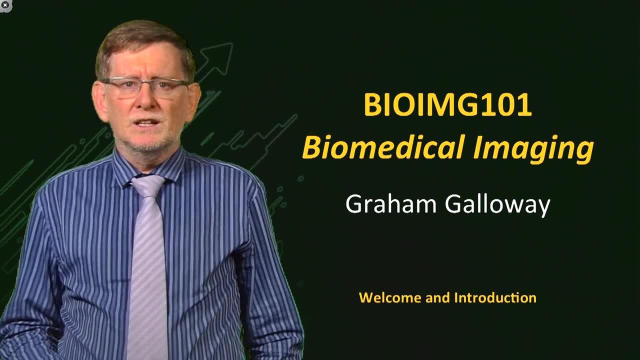 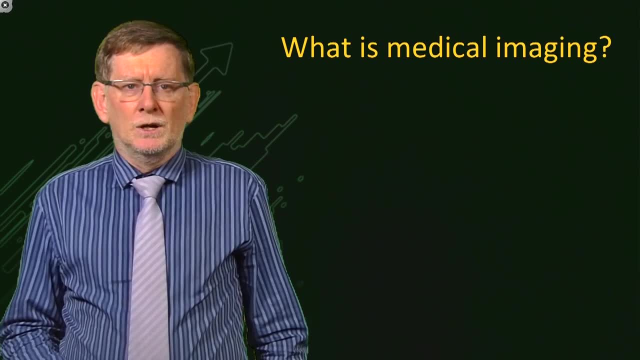 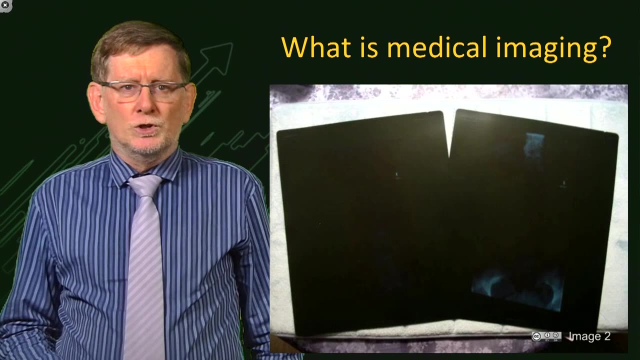 and new ways of using imaging to diagnose everything from simple medical events to complex diseases. What do you think of when you consider medical imaging? To most of you, it is probably those large envelopes which contain sheets of photographic film which you carry from the local radiology centre back to your treating physician. 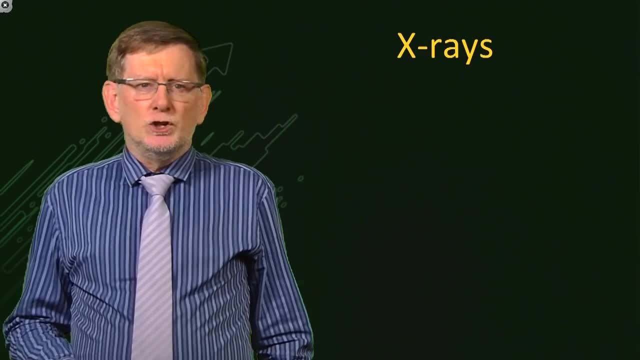 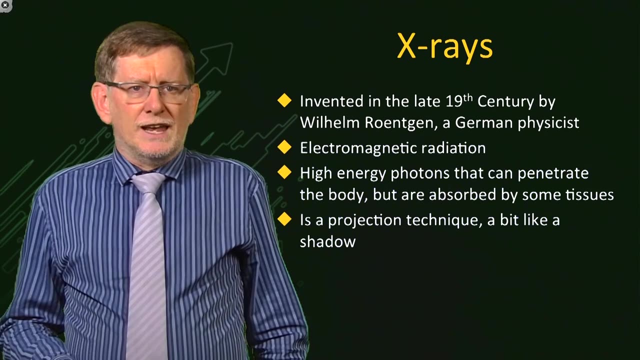 X-rays were invented in the late 19th century by a German physicist, Wilhelm Roentgen. They are a form of electromagnetic radiation and the energy level of the radiation is very high. The energy level of the photons is high enough to penetrate the body. 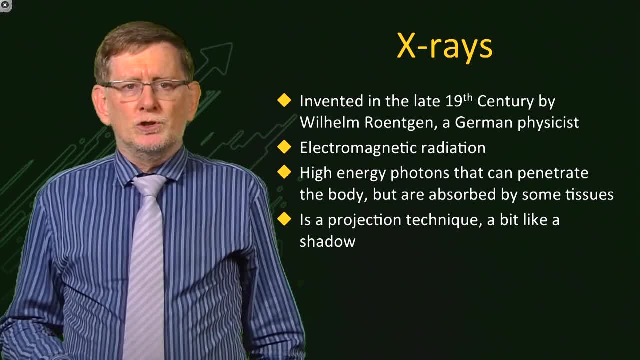 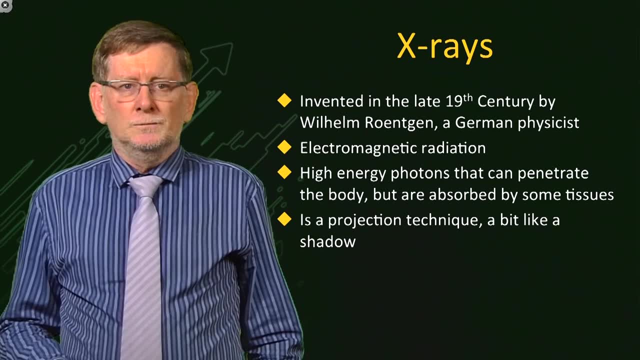 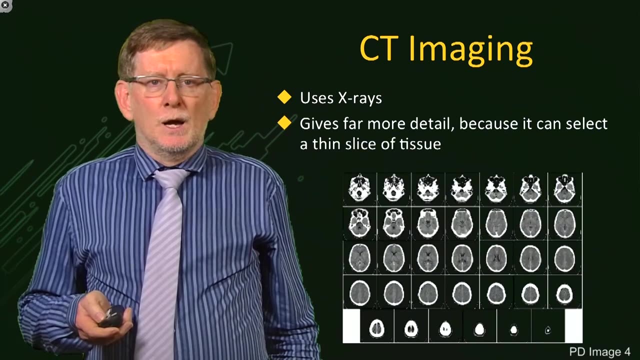 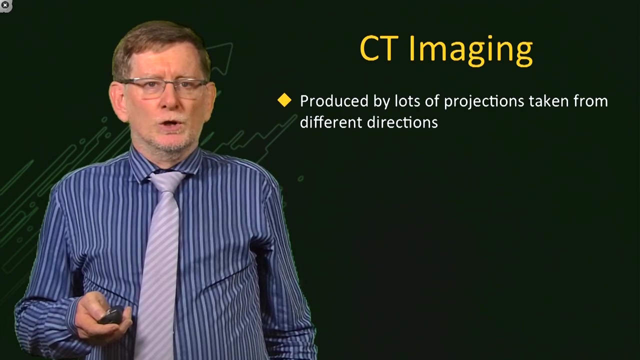 but differential absorption by different tissue types produces contrast. Image production is a projection of the object being imaged, a bit like a shadow. CT imaging also uses X-rays, but it provides far more detail because it is able to select thin slices of tissue. It uses many projections in different directions to build up an image. 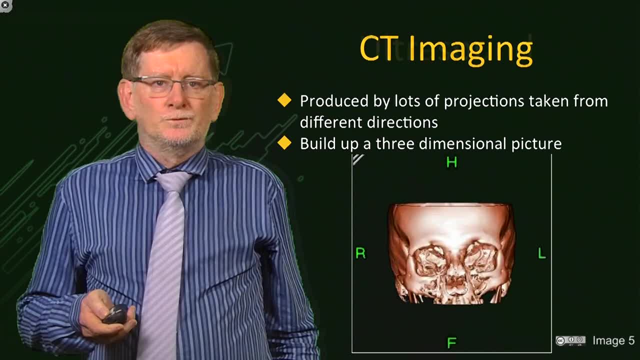 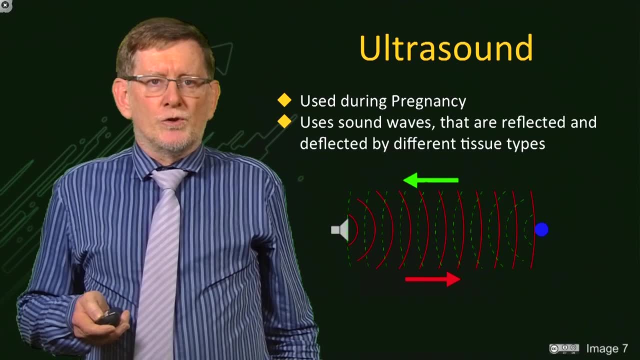 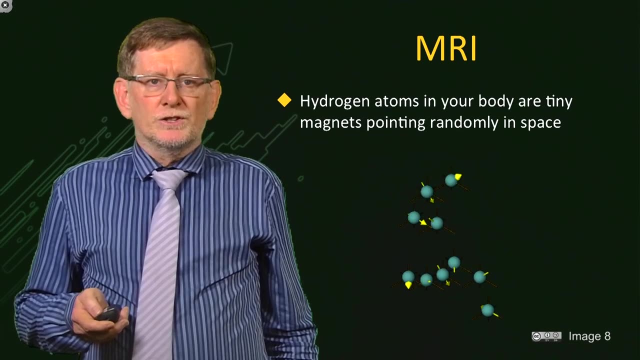 CT can also be used to build a three-dimensional image. Many of you will have had an ultrasound before you were born. The sonographer uses a transducer to transmit sound waves and then collect the signal that is reflected. MRI relies on the fact that in your body, the hydrogen atoms produce a magnetic field. 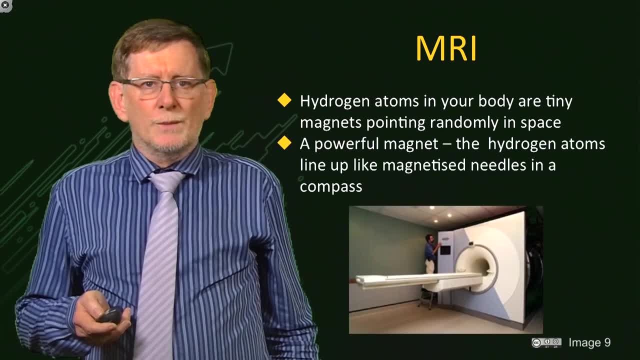 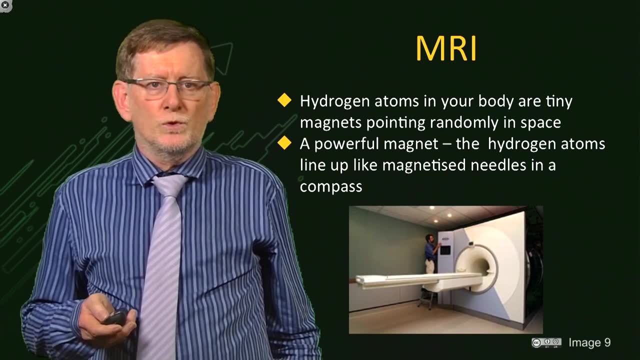 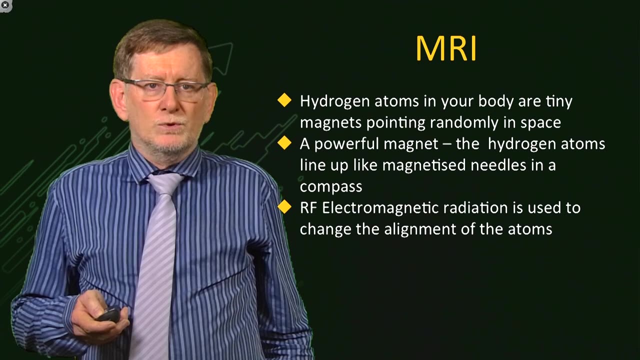 which points in random directions. When they are put in a powerful magnet, they line up in the same way as a magnetised needle in the compass lines up with the Earth's magnetic field. The image changes by simply altering the timing of the acquisition. 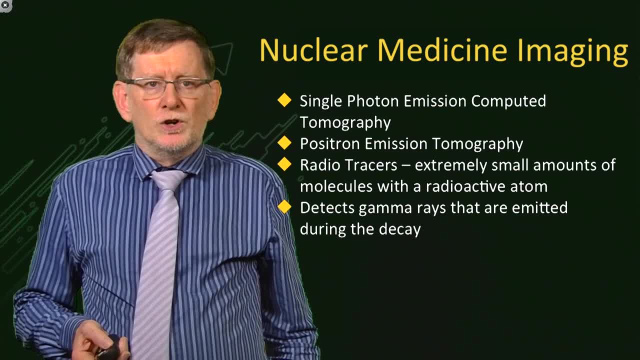 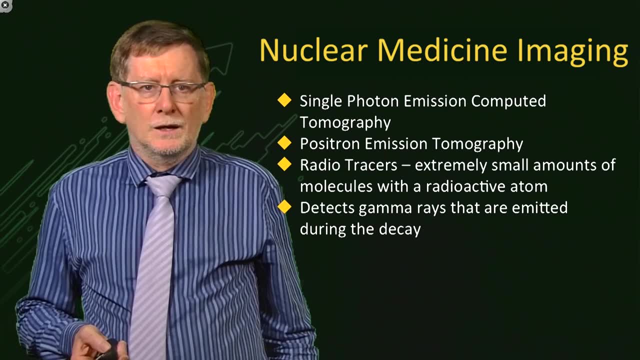 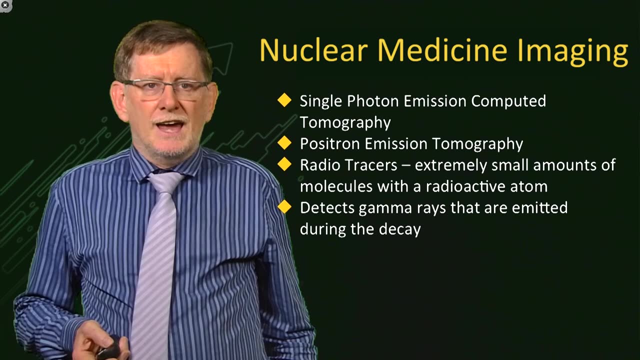 There are two classes of molecular imaging: Single photon emission computer tomography, abbreviated SPECT, and positron emission tomography, or PET. Both use extremely small quantities of a molecule with a radioactive nucleus. The scanner detects the gamma rays, another form of electromagnetic radiation, to build an image.